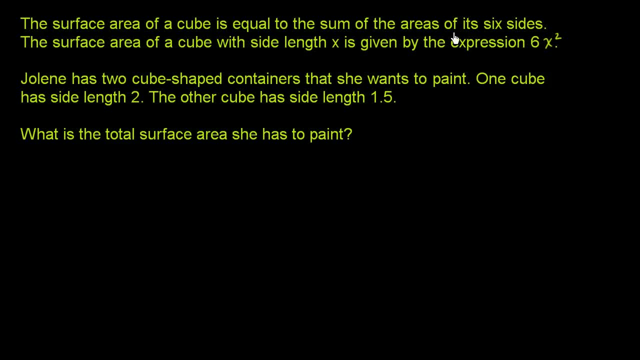 The surface area of a cube is equal to the sum of the areas of its six sides. Let's just visualize that. I like to visualize things. So if that's the cube, we can see three sides. Three sides are facing us. But then, if it was transparent, we see that there are actually 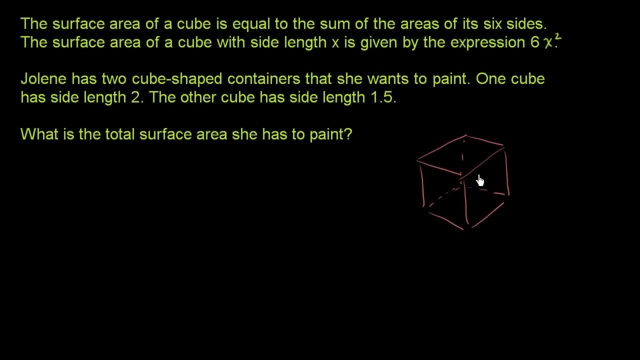 six sides of a cube. So there's this one, one, two, three in front, And then this is the bottom, This is in the back And this is also in the back. So you have three sides of a cube. So I believe what they're saying. 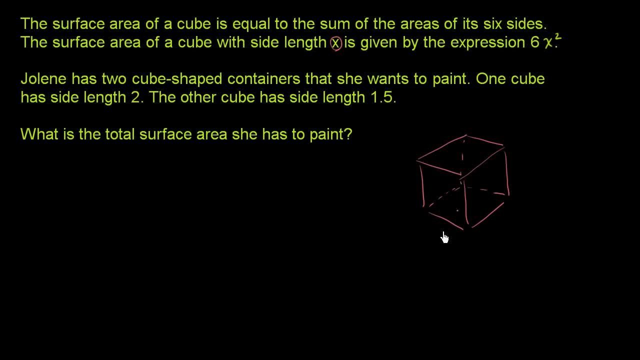 The surface area of a cube with side length x. so if this is x, if this is x, if this is x is given by the expression 6x squared, That also makes sense. The area of each side is going to be x times x. 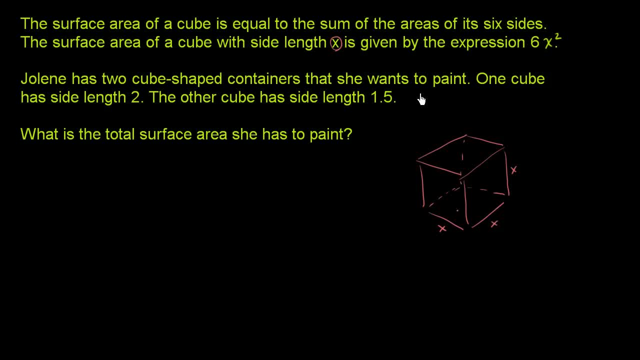 It's x squared And there are six of them, So it's going to be 6x squared. Jolene has two cube-shaped containers that she wants to paint. One cube has side length 2.. So this is one cube right over here. 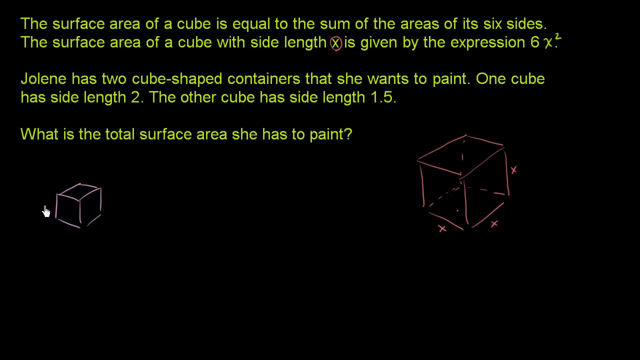 Let me do my best. Let's draw it. So this right over here has side length 2.. So that's its dimensions. The other cube has side length 1.5.. So the other cube is going to be a little bit smaller. 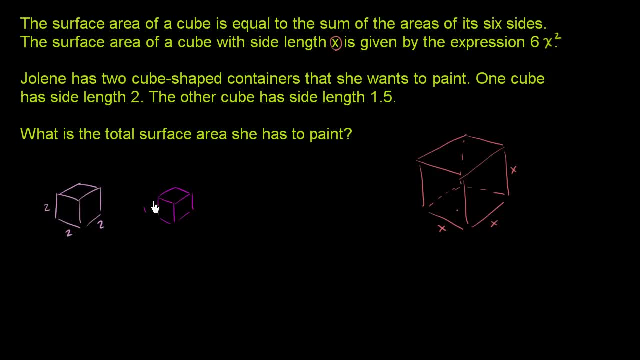 It has side length 1.5.. So it's 1.5 by 1.5 by 1.1.5.. What is the total surface area that she has to paint? Well, we know that the surface area of each cube 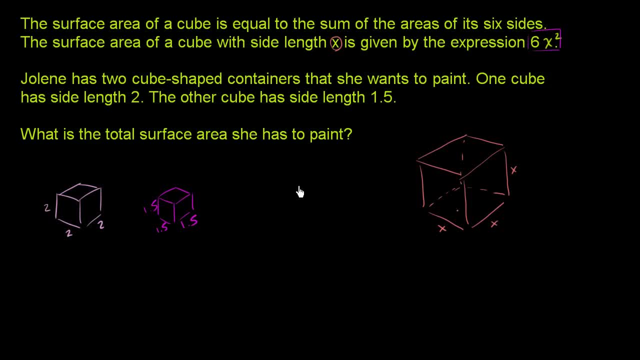 is going to be 6x squared, where x is the dimensions of that cube. So the surface area of this cube right over here is going to be 6.. And now let me do it in that color of that cube: It's going to be 6 times x, where 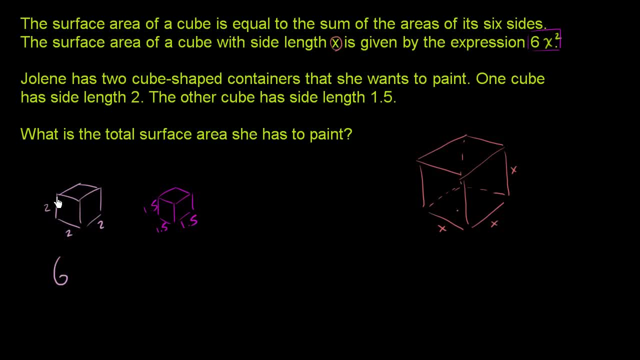 x is the dimension of the cube. And the cube all has the same dimensions, So its length, width and depth is all the same. So for this cube the surface area is going to be 6 times 2 squared, So it's going to be 6 times 2 squared. 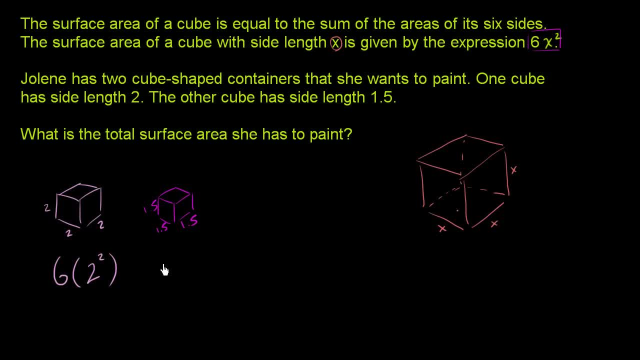 And then the surface area of this cube is going to be 6 times 1.5 squared And if we want the total surface area she has to paint, it's going to be the sum of the two cubes. So we're just going to add these two things.